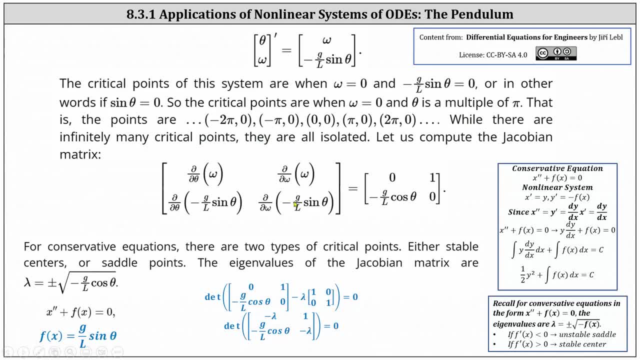 they are all isolated. Next we determine the Jacobian matrix shown below. In the first row we have the partial of omega with respect to theta, which is zero, and then we have the partial of omega with respect to omega, which is one. In the second row, we have the partial of negative g. 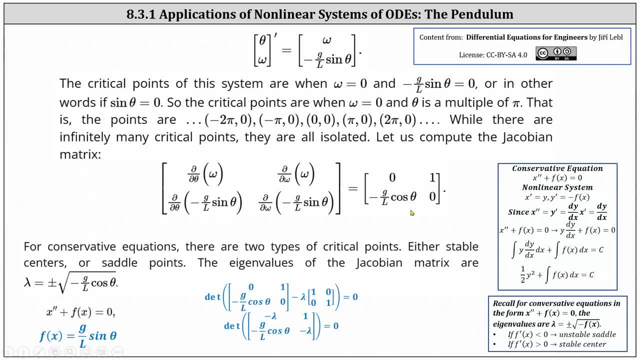 divided by L sine theta with respect to theta, which is negative. g divided by L cosine theta. and then we have the partial of negative g divided by L sine theta with respect to omega, which is zero. Next, referring to our notes below for conservative equations, 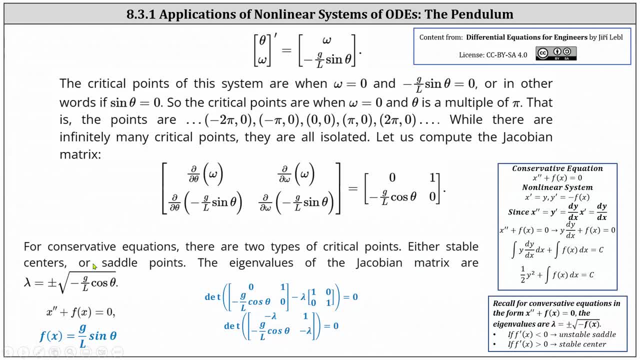 there are only two types of critical points. We either have stable centers or saddle points. We determine which type by determining the eigenvalues of the Jacobian matrix. To do this, we solve the equation below in blue, which results in the eigenvalues. 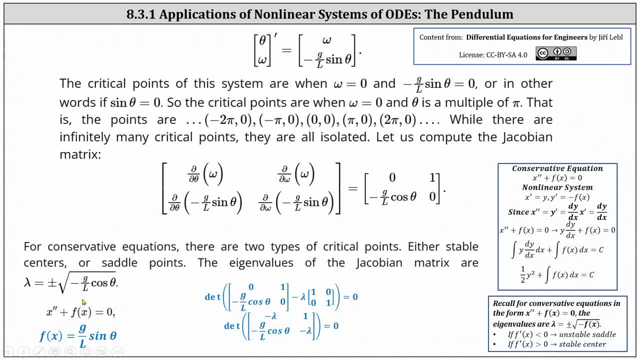 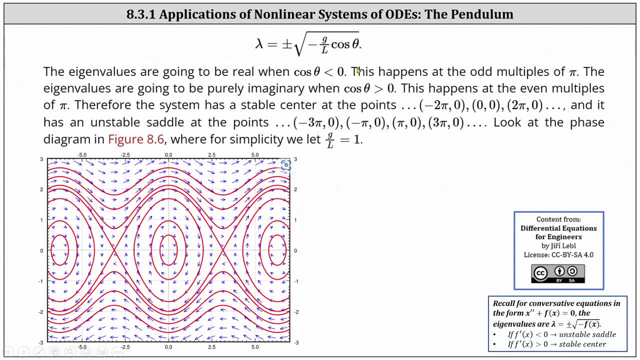 lambda equals plus or minus the square root of negative g divided by L cosine theta. Notice: the eigenvalues will be real when cosine theta is less than zero or negative. This happens at odd multiples of pi and the eigenvalues are going to be purely imaginary. 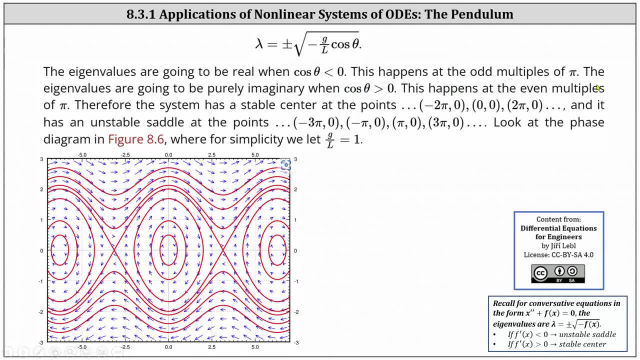 when cosine theta is greater than zero or positive. This happens at even multiples of pi. Therefore, the system has stable centers at the points dot, dot, dot. negative, two pi, comma zero, zero, comma, zero, two pi. 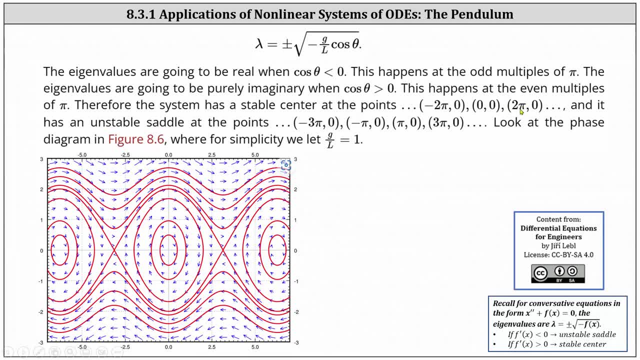 comma zero. dot dot dot, where theta is an even multiple of pi And it has an unstable saddle at points. dot dot dot. negative three pi. comma zero, negative pi. comma zero pi. comma zero three pi. 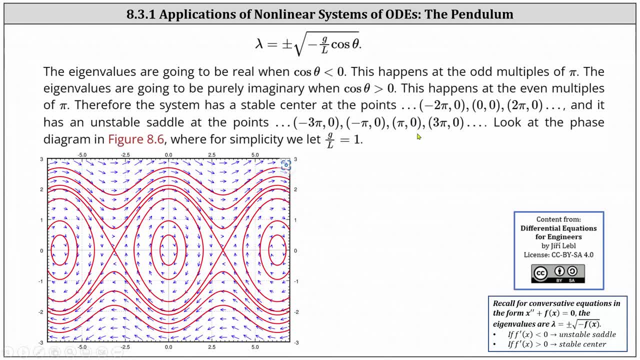 comma zero, dot, dot dot, meaning when theta is an odd multiple of pi. Below we have the graph of the phase diagram where, for simplicity, g divided by L is equal to one. Notice we do have stable centers at negative two pi. 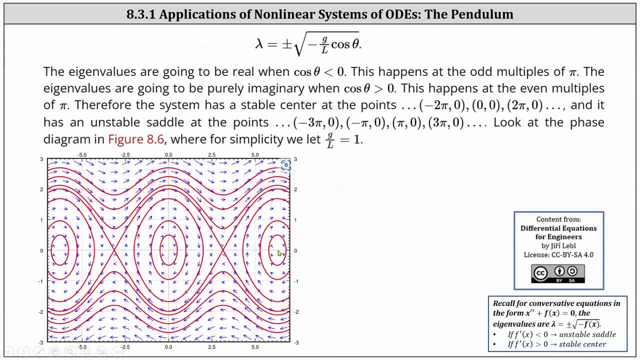 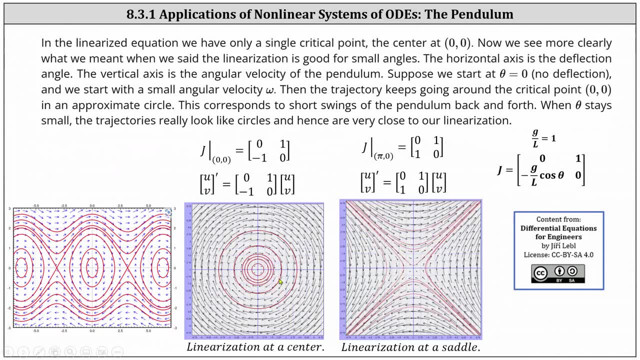 comma zero, zero comma zero and two pi comma 0 and we have unstable saddle points at negative pi comma 0 and pi comma 0.. Looking at the looking at the phase portraits, below on the left we have the phase portrait for the original. 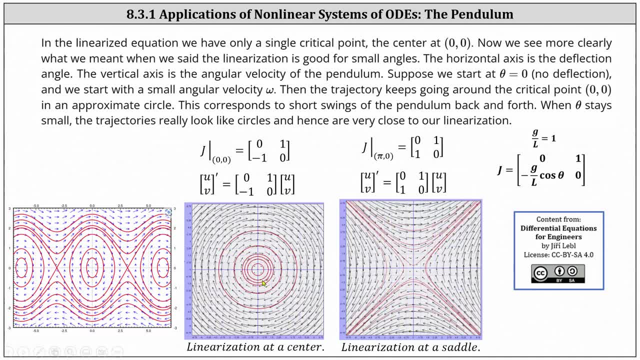 system. Next, we have the linearization at the point 0 comma 0, where we have a stable center, and on the right we have the linearization at the saddle point pi comma 0.. Let's focus on the phase diagram and the linearization at the point 0 comma 0.. In the linearized equation we have only: 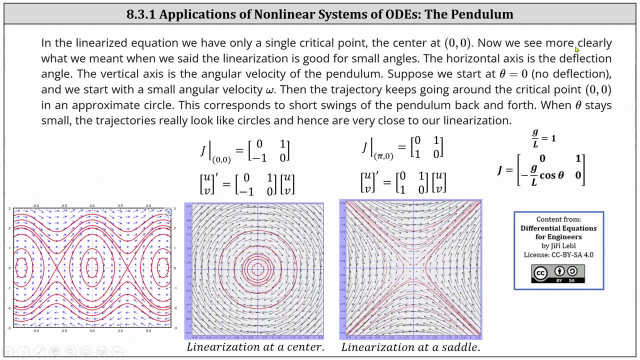 a single critical point: the center at 0 comma 0.. Now we see more clearly what we meant when we said the linearization is good for small angles. The horizontal axis is the deflection angle and the vertical axis is the angular velocity of the pendulum. Suppose we start at, theta equals 0. 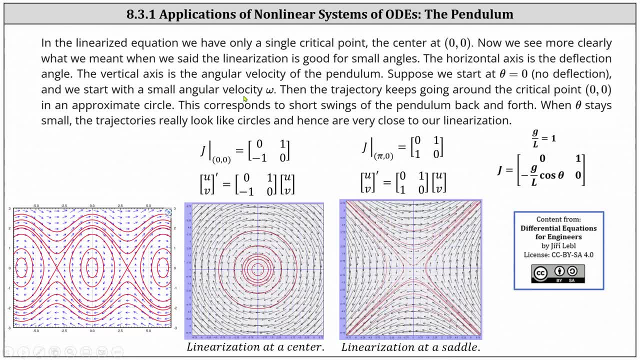 meaning no deflection- and we start with a small angular velocity, omega. Then the trajectory keeps going around the critical point 0 comma 0. This corresponds to short swings of the pendulum back and forth. When theta stays small, the trajectories really look like circles and hence are very close to the linearization When we give 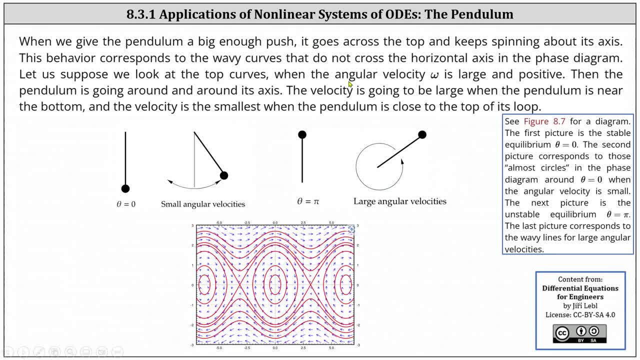 the pendulum a big enough push. as shown here on the far right, it goes across the top and keeps spinning around its axis. This behavior corresponds to the wavy curves that do not cross the horizontal axis in the phase diagram. Supposedly look at the top curves. 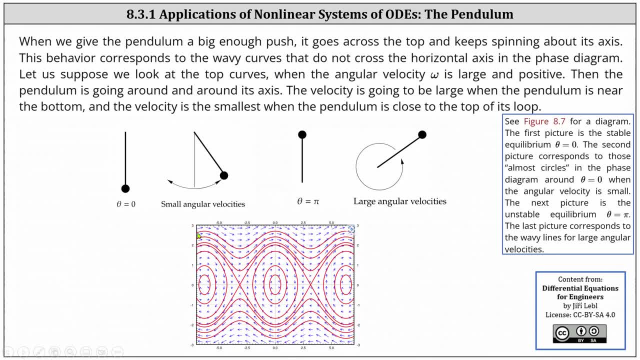 which are the horizontal axis and the phase diagram. If we look at the top curves, we see that when the angular velocity, omega, is large and positive, For example along this trajectory here, Then the pendulum is going around and around its axis. The velocity is going to be large when the 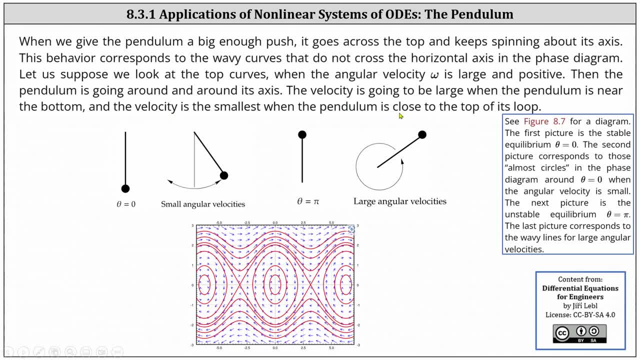 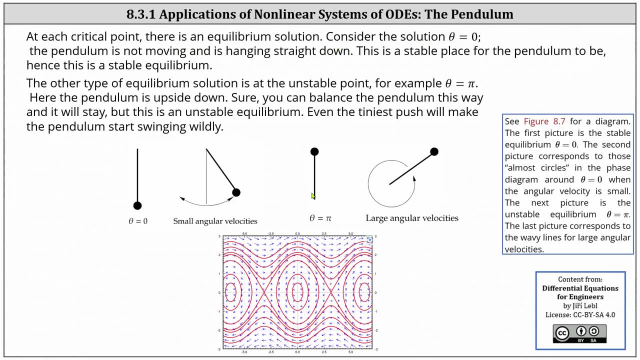 pendulum is near the bottom and the velocity is smallest. when the pendulum is close to the top of its loop, At each critical point there is an equilibrium solution. Consider the solution theta equals 0 shown here on the left. The pendulum is not moving and is hanging straight down. 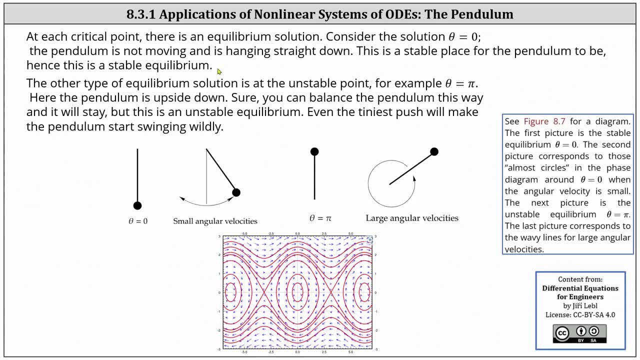 This is a stable place for the pendulum to be. Hence this is a stable equilibrium. The other type of equilibrium solution is at the unstable point. for example, theta equals pi, shown here. Here the pendulum is upside down. Sure, you can balance the pendulum this way and it will stay, but this is an unstable equilibrium. 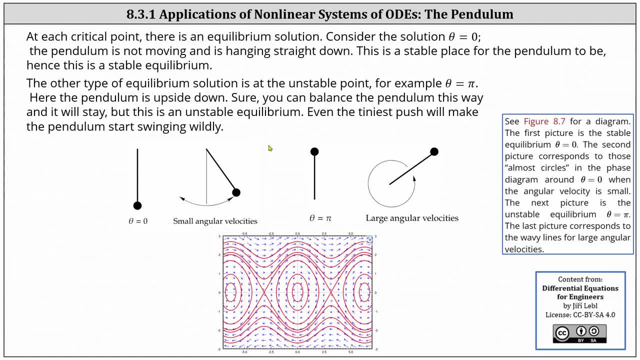 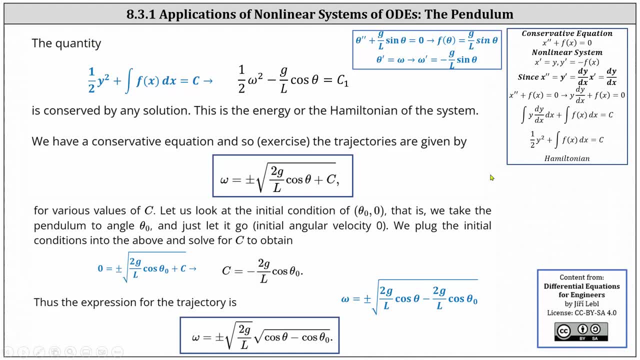 Even the tiniest push will make the pendulum start swinging wildly. And now let's go back and work on determining the equation of the trajectories. Because we have a conservative equation: the Hamiltonian, or one half y squared Plus the integral of f of x, dx equals c, is conserved by any solution. 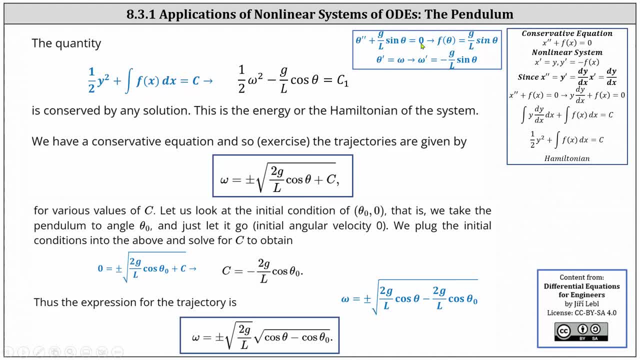 Or if we go back to the pendulum equation, Notice our function: f is f of theta equals g divided by l sine theta, And the integral of g divided by l sine theta with respect to theta is negative g divided by l cosine theta, And therefore the Hamiltonian is one half omega.